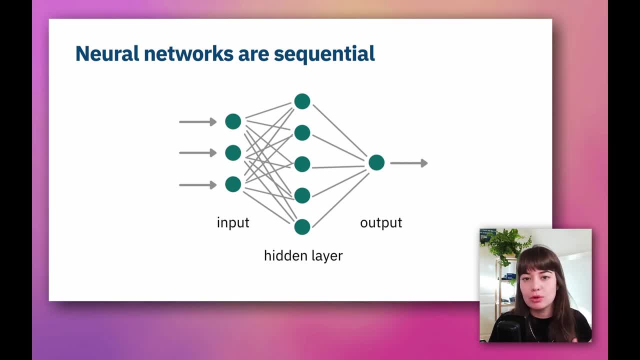 So, if you remember, in a normal neural network- or a deep neural network, you can call it- we have an input layer, a hidden layer and an output layer, And information runs sequentially. So first the information comes to the input layer, then it is passed to the hidden layer. 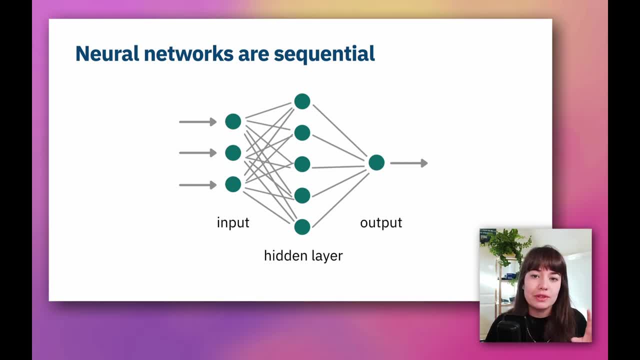 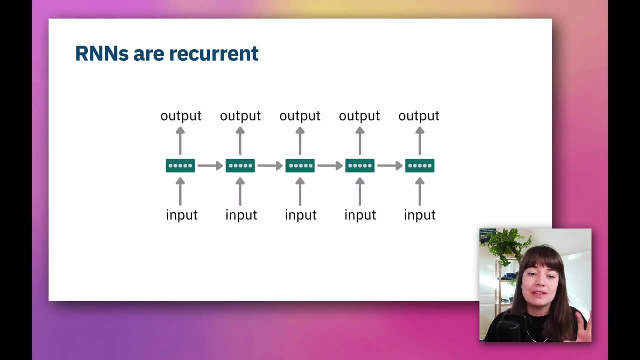 and then, finally, the output is produced. So all of the data points that you have, you give them at the same time, all of the features of your specific data point that you're training on. The difference in neural networks of recurrent neural networks is that 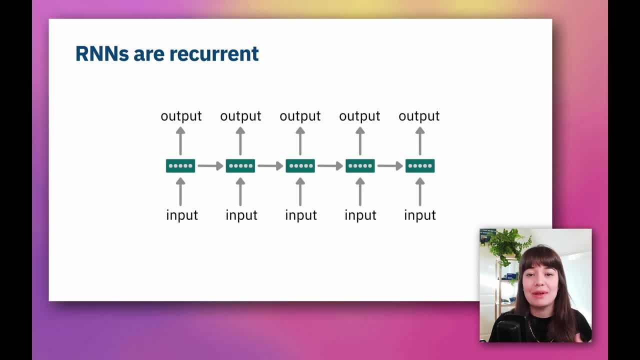 they are recurrent, So that means that the same thing happens over and over again, in a way. So this is what a recurrent neural network looks like when it's unrolled, And I will also show you how recurrent neural networks look like when it's unrolled. 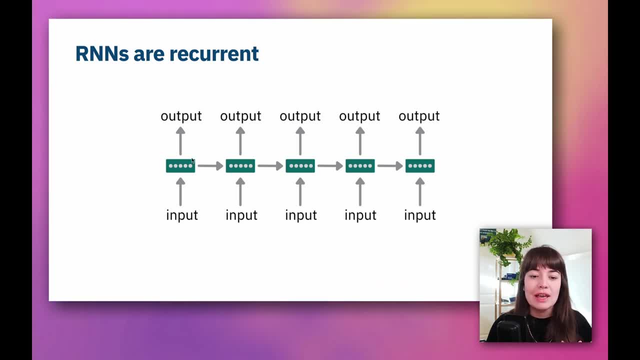 But basically, what you need to know is that each of these little sections are actually one of the same. They're the same network or they are the same neurons. So what happens is these are all the different input features and you give them one after another. So you first. 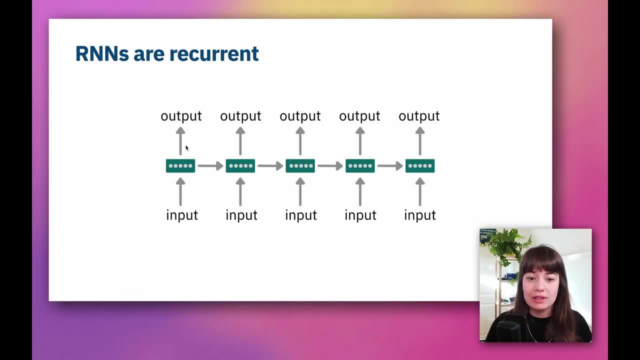 give the first feature of your input and output is calculated and also pass to the second time step- We call them time steps- And then the second feature of your input- data input or a data point is given, including the output of the first one. 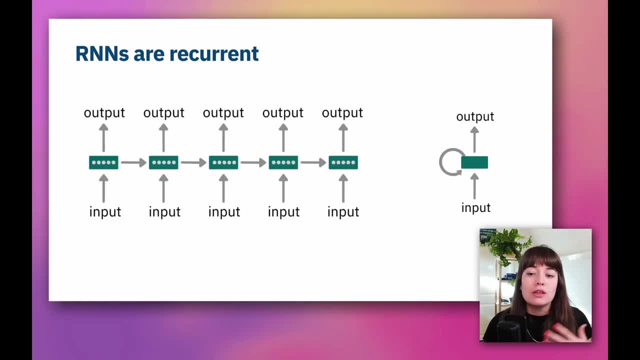 another, output is calculated, and so on and so forth. So when you put it, when you show it as it is actually and how it is, is that it is just one unit. So what happens is you give it an input, output is calculated, but at the same time output is passed again. the second feature of the input: 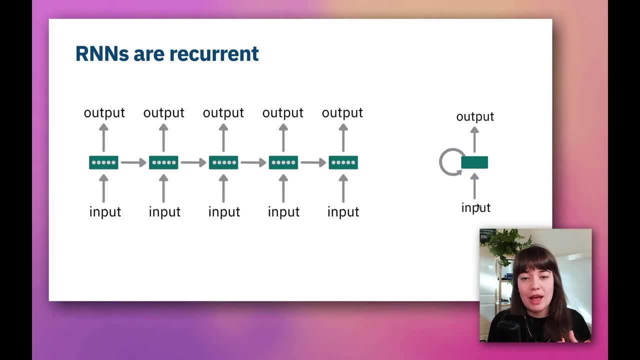 is given. So when you compare it to neural networks, what happens is in neural networks you give all of the features at the same time, whereas in the current neural networks you give all of the features one step at a time. So it is basically: things happen in a time step manner. So we would call this the first time. 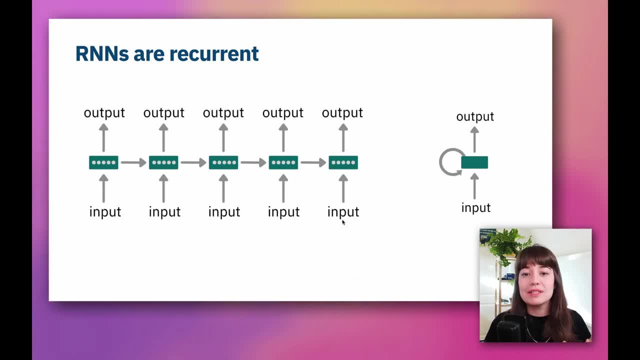 step, the second time step, third, fourth and fifth time step. So, basically, in each of these time steps, except the first one, you have two inputs. One of them is the output from the previous time step and one of them is the input of this time step. So how do we calculate the output of? 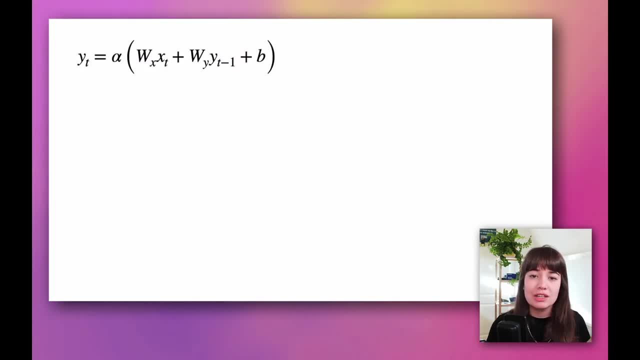 recurrent neural networks. Well, we do it with this formula. It's actually quite simple, even though it looks like a complication. So we do it with this formula and it's actually quite simple, even though it looks like a complication. So we do it with this formula and it's actually quite simple. 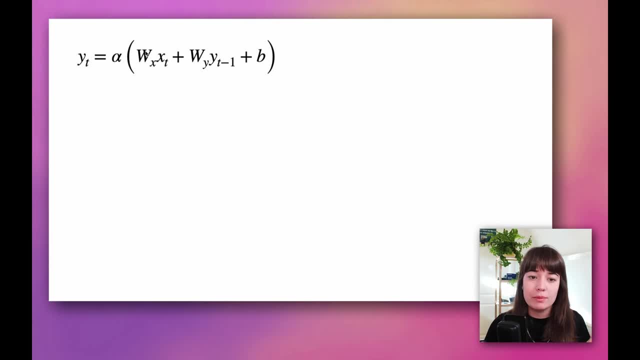 math formula thing. You have weights for your inputs. So for each time step you have the weights, And for all of the outputs from the previous step you have another set of weights and you also have the biases. All of this is of course passed through an activation function. 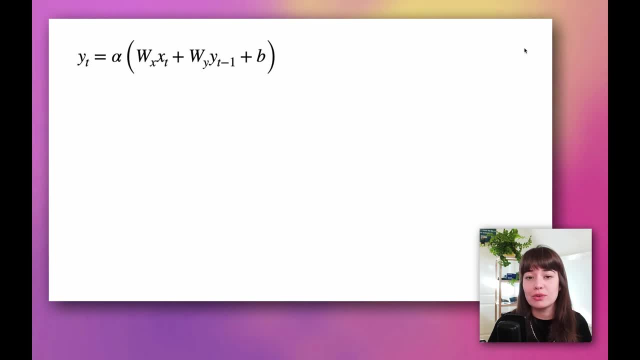 and at the end you have the output of your recurrent neural network. One thing to understand here is that, even though it looks like we have many steps, as I said, it's actually just one unit. So wx and wx are the outputs of the recurrent neural network, So we have the output of the 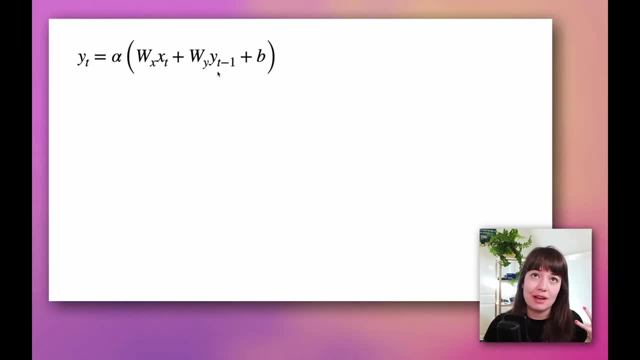 wx, which are the weights of the output of the previous layer and the input of this layer, or time step, is the same, because they're actually the same Here. we're just showing them in an unfurled way because it's easier to understand. So there's only one set of weights for the input. 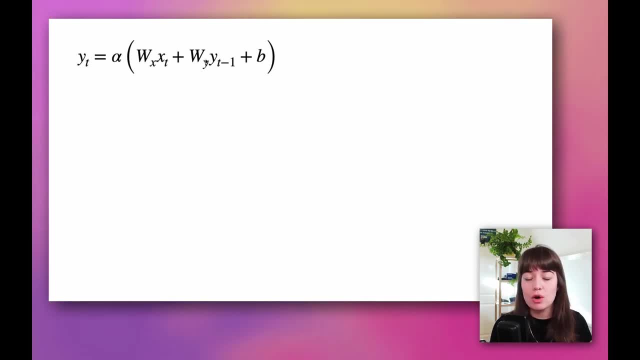 and one set of weights for the output. So there is a very common way of showing cells of RNNs. because these cells- here how the output is calculated- can be different And we will talk about different types of cells too. But let's talk about how to depict a simple RNN cell. 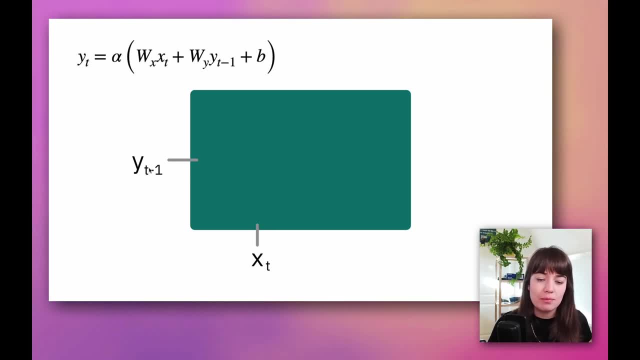 So what we normally have, of course, as we talked about the input, the output from the previous step time step and the input of this time step. So these t's basically depict this time step, t's, This time step. t minus one is the previous time step. So to show this formula on a diagram, 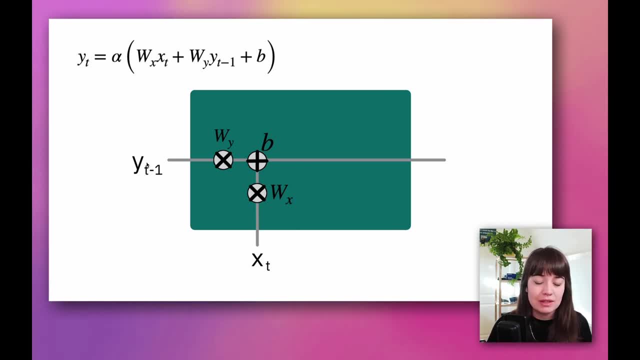 we can say: okay, there is a multiplication happening here, This is multiplied with wy, and here another multiplication, and this is multiplied with wx, And then we also add the bias here. So that's why you know the crosses and the pluses here, And this all goes through an 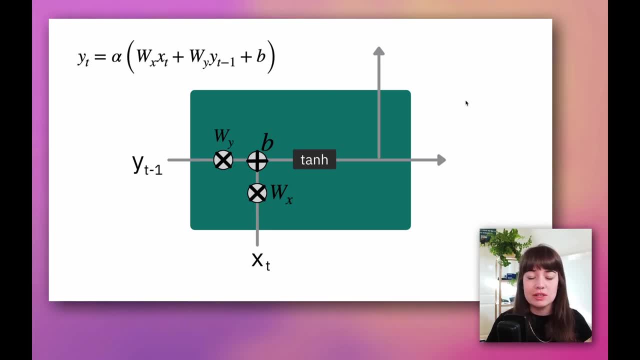 activation function, of course, And very commonly what's used is the hyperbolic tangent function, But of course you can use other things too. But generally hyperbolic tangent function is the one that is being used with simple RNNs And at the end we pass the output of this time. step to the 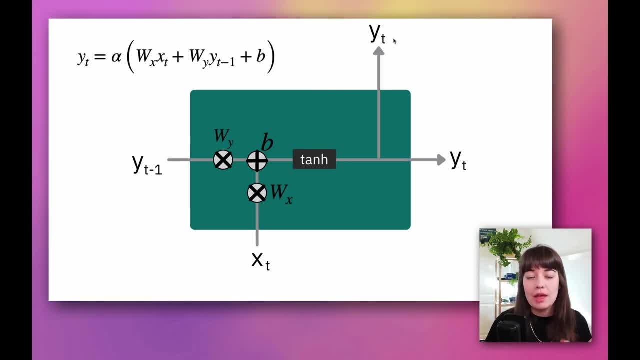 next time step and also we output it. But sometimes this is not the case. So for simplest of RNN cells this is the case where you pass the output to the outside world and also to your next time step, But sometimes you 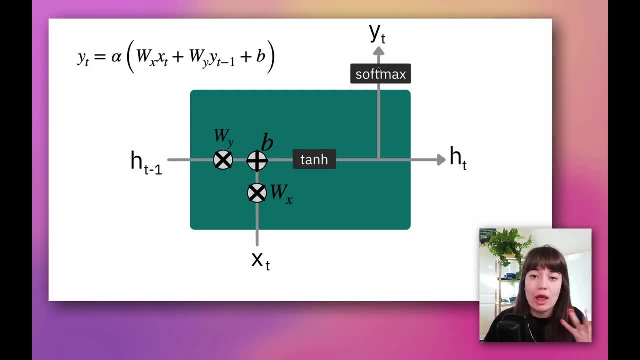 do an extra step on before you output something. So you maybe pass it through a softmax function if you want it to be between zero and one instead of minus one and one, because that's what the hyperbolic tangent function will produce. Then, basically, what you pass to the next state will. 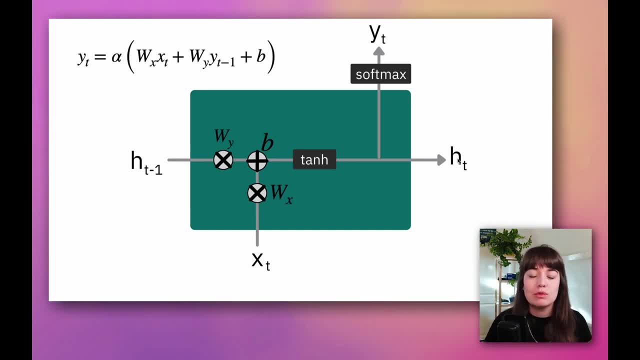 not happen. So you have to do a whole new step. So for the next time step, you pass it through, go through the softmax function, that extra step, and then it will still pass it to the next function or next time step. so it still is the same thing but has seen less processing. so then what happens? 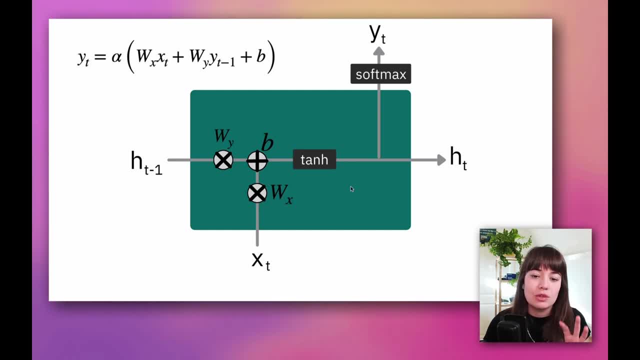 is we call this the hidden state of this time step. so the hidden state of this time step is passed to the next time step. so this is just a interesting difference to keep in your mind that you do not always just pass the output that you get to the next time step, but sometimes we call: 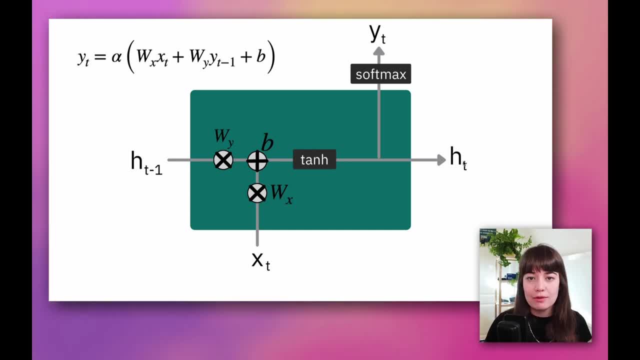 it the hidden, hidden state. there are, of course, a bunch of ways how you can use this architecture, because you do not always have to pass all of your or output all of the outputs that you calculate in your cells. so let's look at a couple of different options. the first type is sequence to sequence. 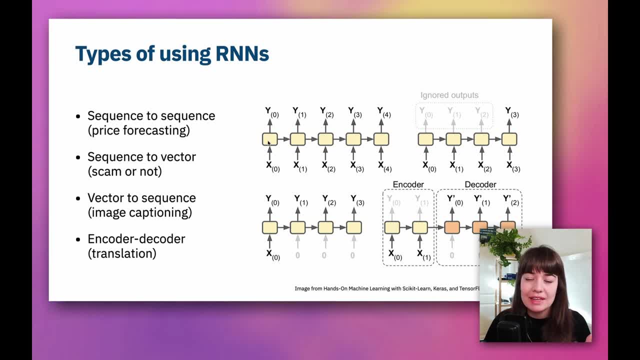 rnn model. so basically, for every input that you give in each time step, you get an output for that time step and for these kind of things. you can use for things that where you're forecasting things, so for example, price price forecast or stock exchange forecasting sort of things. uh, the second one that you can use is called 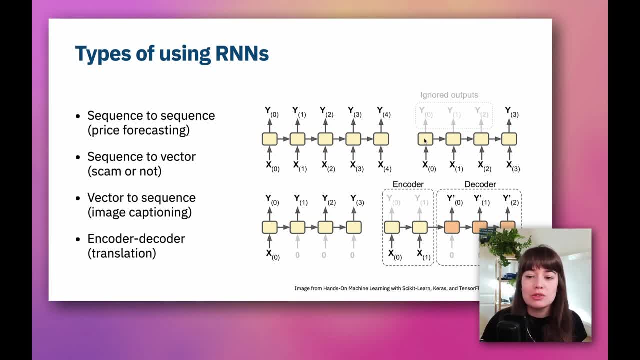 sequence to vector. sometimes it's called sequence to single, because you only get one output at the end of the whole rnn network that you have um and these things that you use for. let's say, you have a sentence or you have an email, and at the end of the or as an output of the model, what you want. 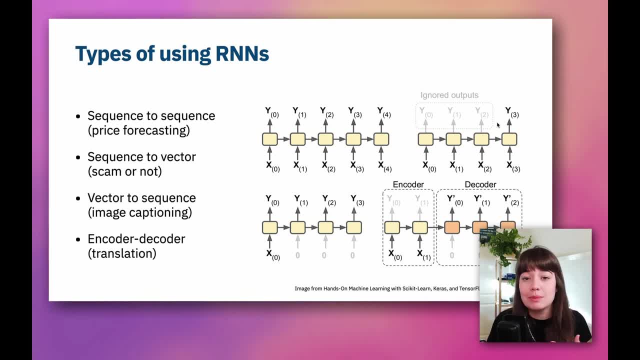 to know is: is it scam or not? or, for example, sentiment analysis, like: what kind of sentiment does it have? is it negative, positive, that kind of things. so for that, in each time step, you give your network a input and then you just ignore the outputs. even if it's producing the outputs, you do not look at them, the only output. 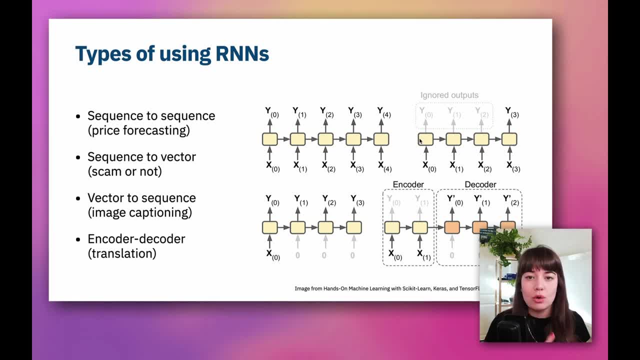 that you look at is the one at the end, because before seeing the whole sentence, your model cannot come to a conclusion. of course, another one that you have is vector to sequence or, as I said, single to sequence. by the way, the reason that they are not called single but vector here is that because 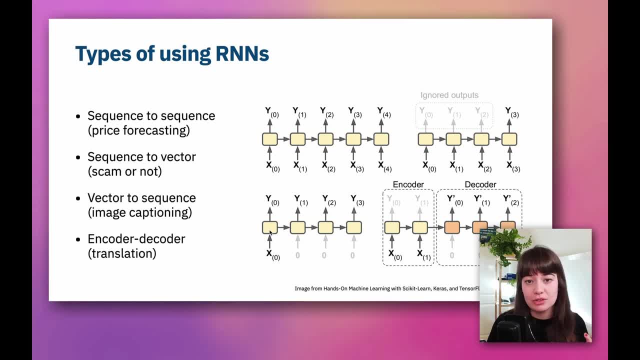 the output that you have is in the form of a vector most of the time, and it is not just a single number. that's why we just call it vector instead of single, but both ways are fine. so in vector to sequence sort of architectures, what you're doing is you're giving the network one. 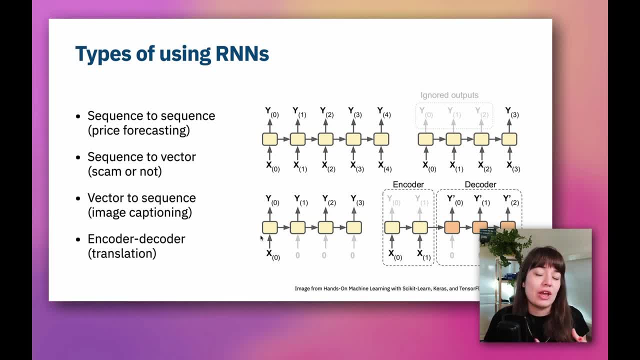 input and you are letting it output a sequence of things. so this could be: for example, you give your network an image and then you're having it output a explanation of that image word by word. so let's say, you give a photo of a dog running on a beach, then for each of these time steps the network will output a dog. 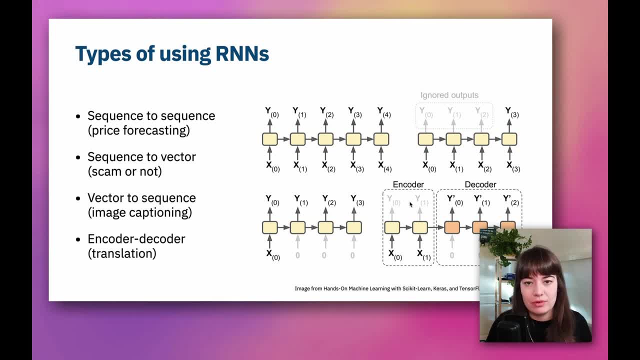 running on the beach, for example. so those are the kind of things that you would use a vector to sequence architecture for. and lastly, we have encoded decoder sort of architecture. so in these kind of architectures- RNN architectures- at first you are only giving your network inputs, so input. 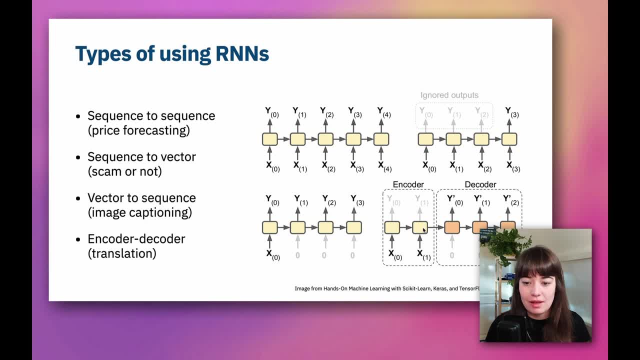 input: input for a couple of time, steps or how many ever that you need, and then you get outputs. so, and then in the second part, you only get outputs, you do not give any inputs. and these kind of architectures are good for translation, because to translate a sentence, your network needs to see the whole sentence. words, because 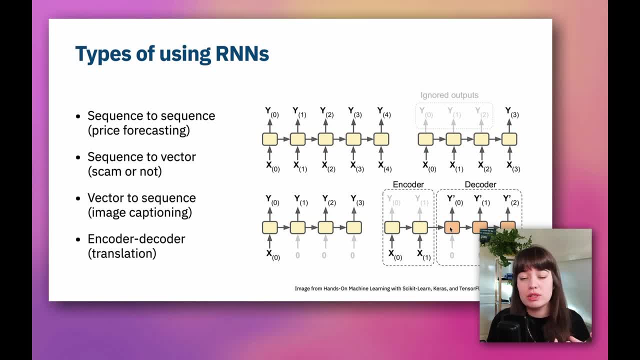 meaning of some words might change. the translation of some words might change if you see the whole sentence based on the context. so that's why you first give it the whole sentence and then you get the translation word by word. on the decoder part, all right, but how do you do that? 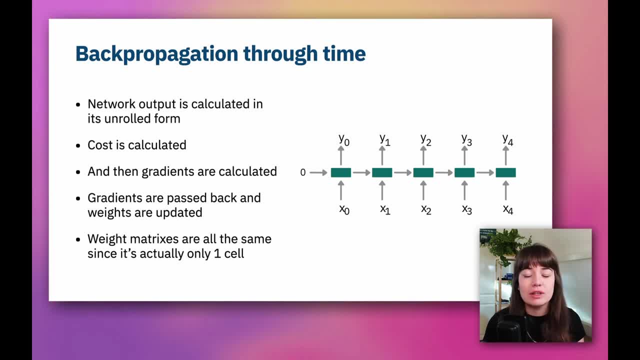 how does RNNs learn? so how does the training work? it's actually quite simple. it's very similar to normal neural networks that do not have any interesting architecture, but we just call it back propagation through time. so what happens is the output of the network is calculated, of course. 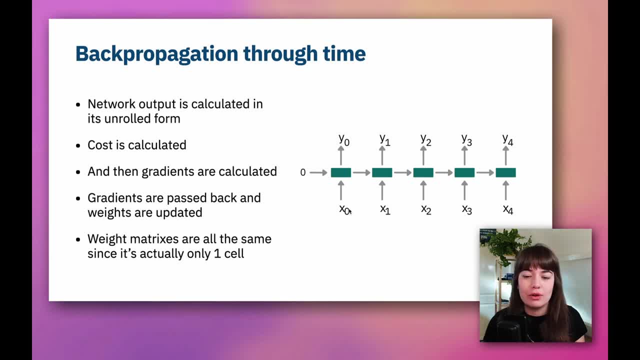 and we do it in. you can think of it as like it's unrolled for a form, so at first you give it input as zero, and then or the hidden states from the previous state, and then you give it input as zero, and then or the hidden states from the previous state, and then you give it input as zero, and then 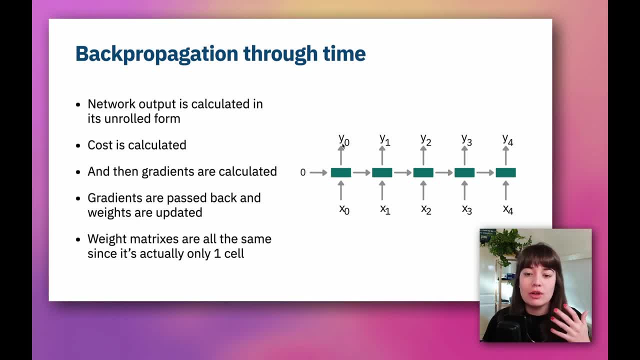 if you wanna figure out what two outputs are and then considering until we had this time set, because it doesn't exist as zero- you give the first input, you get a first output, you give the second input, you get a second output and then you just calculate which, whatever. 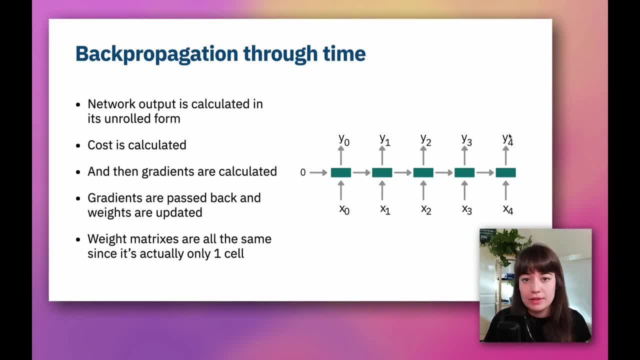 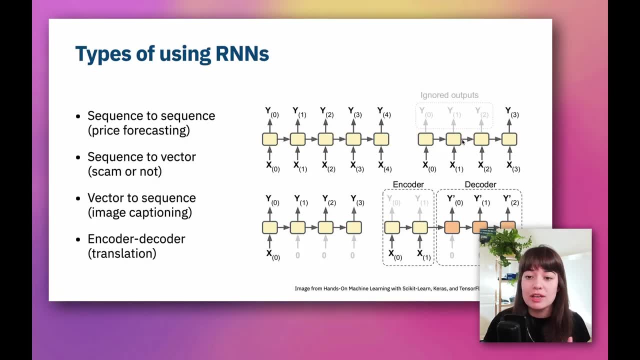 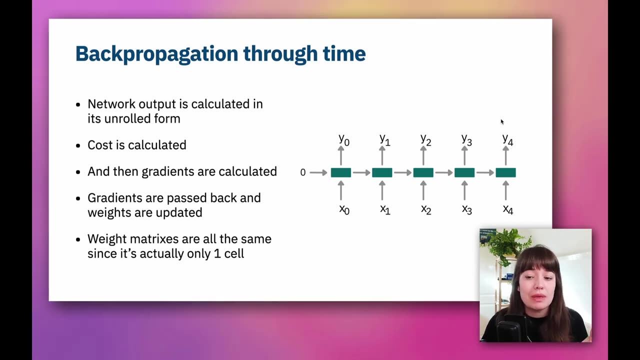 you want to calculate and then we calculate the cost of this network. but, as we said in the previous slide, sometimes the network how you use the network. so you might want to ignore the first couple of. maybe you're just interested in the last two outputs or maybe even you're just interested. 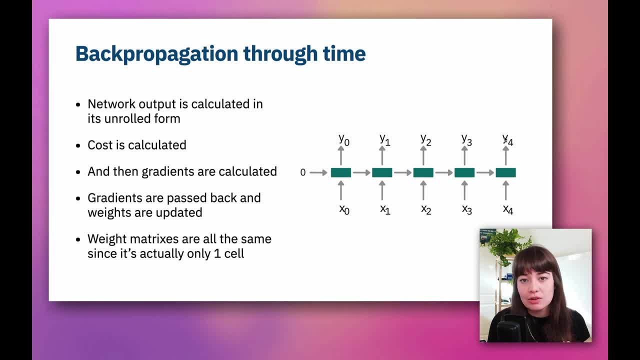 in the last one. so, based on that, cost is calculated And then, based on that, as we did with normal neural networks, we calculate the gradient and then the gradient is passed back through the network and the weights are updated. But, as we said, all the weights of all of these time steps are actually the same, because they're 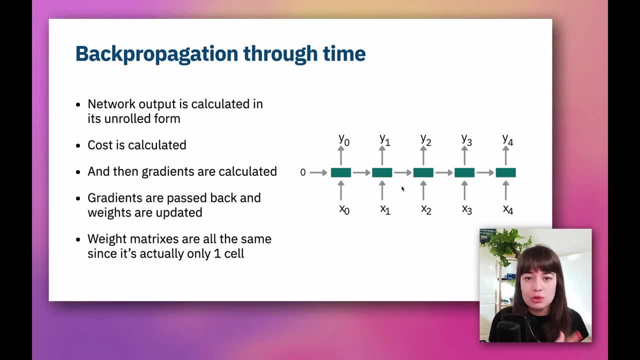 actually one time step, And then the gradients are calculated as we do with normal neural networks, And then these gradients are passed back in the network to update the weights, But, as I said, you might ignore some of the outputs while you're calculating costs. So the gradients are. 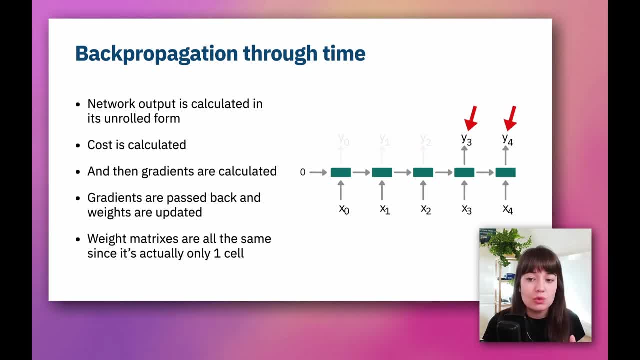 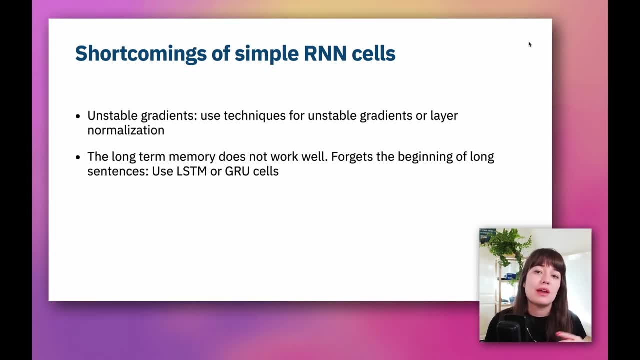 passed back only through the ones that you used in the cost calculation. So RNNs are actually really good for analyzing sequential data, So this could be time series, data, text or audio files, for example. But of course they have some shortcomings. So the first one is that they have unstable 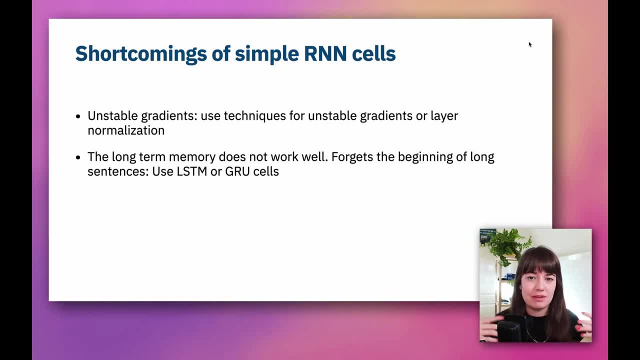 gradients And you can imagine that right, Because it's a very long sequential sort of architecture. The further back you go in this architecture, the smaller your gradients are going to get. So you might not be able to update the weights on the previous time stamps in a way, or to previous time steps in a way. 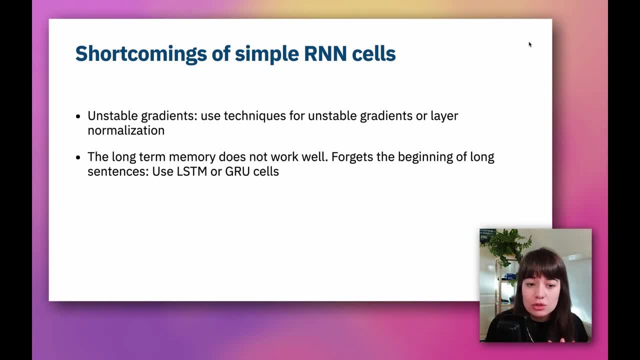 that will be helpful for the whole network. What you can do for this problem in RNNs is use other techniques that we use for normal neural networks too, or just deep neural networks too, to deal with unstable gradients. Or you can use layer normalization instead of batch normalization. 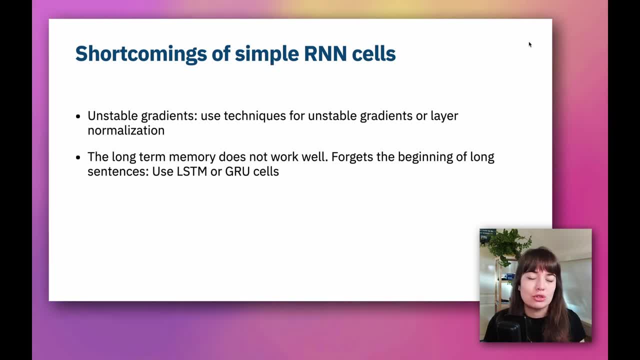 because batch normalization is not as effective. It's recurrent neural networks, So they're kind of tricky to apply to recurrent neural networks, So instead you can use layer normalization. And another problem with simple RNN cells is that they forget. If you give it a very long sentence it tends to forget what was being said at the 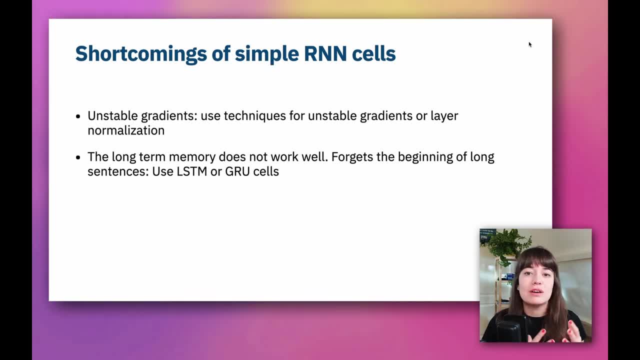 beginning of the sentence. So the applications that are created with it are not really effective or they don't work as well. So instead we have the LSTM or GRU cells that we can use to make sure that we get the meaning of a sentence at the end of it. So let's see what a LSTM cell looks like. 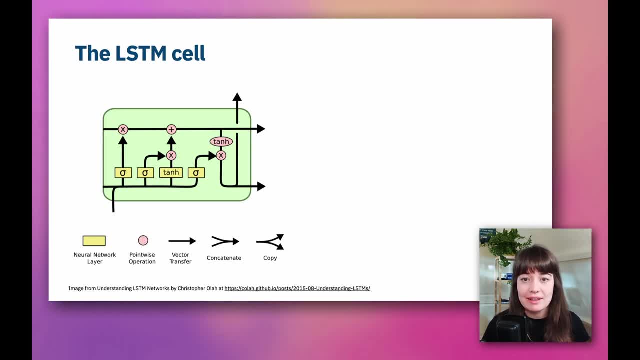 If you remember how I showed you in that diagram the RNN architecture, the simple RNN cell, looks like, it will be easier to understand this one here. So what we have is a couple of sigmoid activation functions And then we have another hyperbolic activation function, And you know. 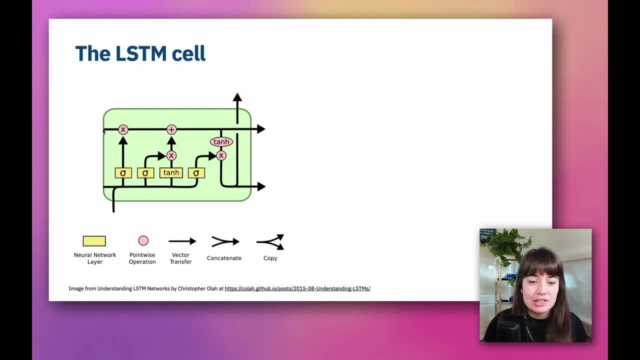 we here see that there are two hidden states that are passed from the previous time step to us And again pass those two different hidden states to the next time step, And then we again have an input and then we have an output. So let's look closely what all of these things mean. So the 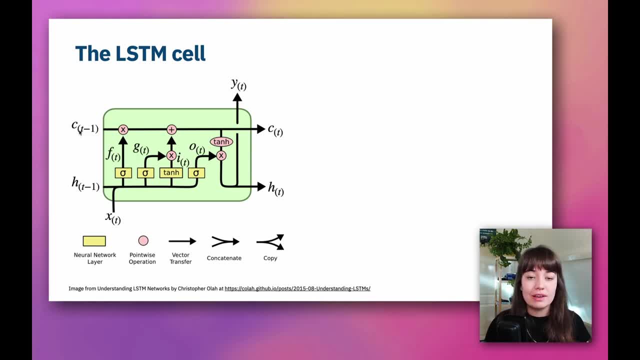 first thing that we need to understand here is that, as I said, we have two hidden states coming and going to the previous and next time steps. The first one is the previous one, as we talked about. it's just a hidden state from the previous step, But the other one, C is a long term memory. 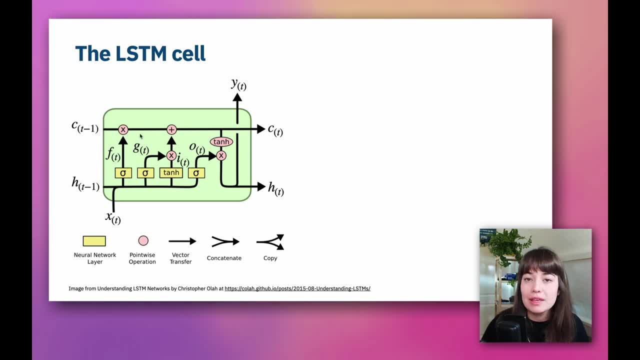 hidden state. So basically, as you say, are less things happening to this hidden state And we either forget or add some things to this long term hidden state and it passes to the next time step without much coming out of it or going into it. Why do I know or how do I know things are being added or extracted from these time steps? 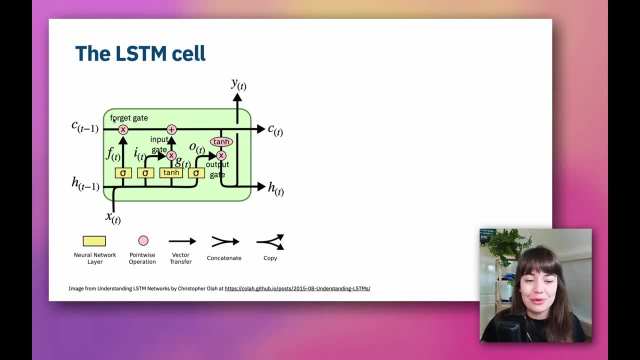 Well, because we have the forget gate here, we have the input gate here and we have the output gate here. So basically, these are the gates that create the information workflow or the how this information is used in this specific time step. So let's talk a little bit more in detail about that. So what we have here are called 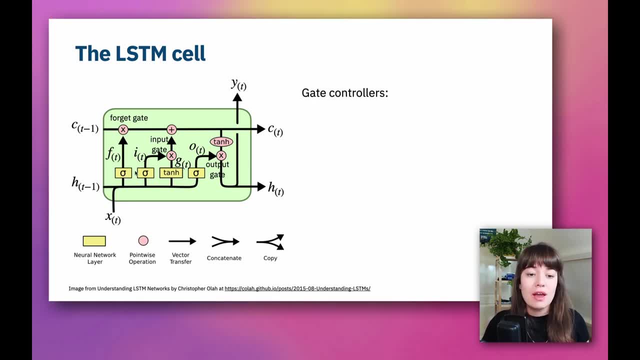 gate controllers, So anything other than the hyperbolic tangent function we call the gate controllers. And what the gate controllers do is they either input zero or one, And in this way they determine if something is going to be forgotten, if something is going to be input or 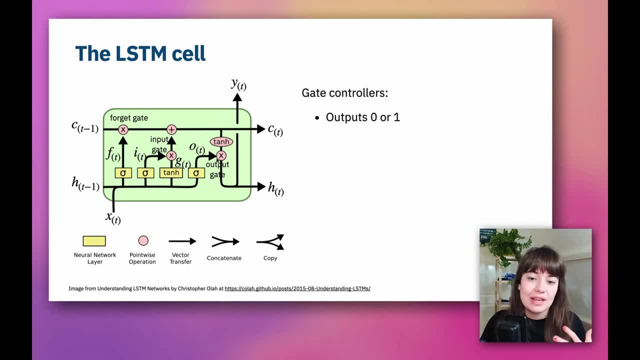 something is going to be forgotten, And then they determine if something is going to be forgotten, if something is going to be output from the long term state And how this works is basically in the forget gate. we decide which part of the long term memory should be removed from the long term. 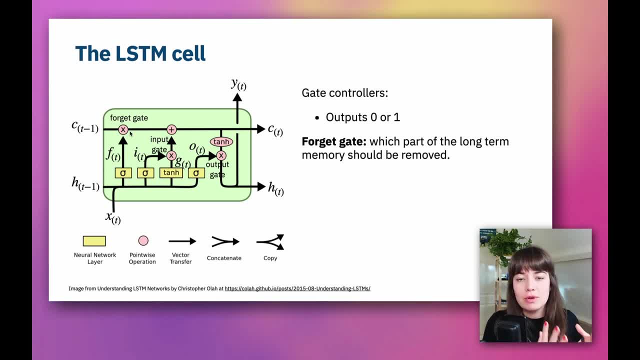 memory. So you know we're saying, OK, this can be forgotten, now We don't need to understand, We don't need to remember this information anymore. In the input gate we decide which part of the hidden state or the information that we just added to the hidden state needs to also be passed on to. 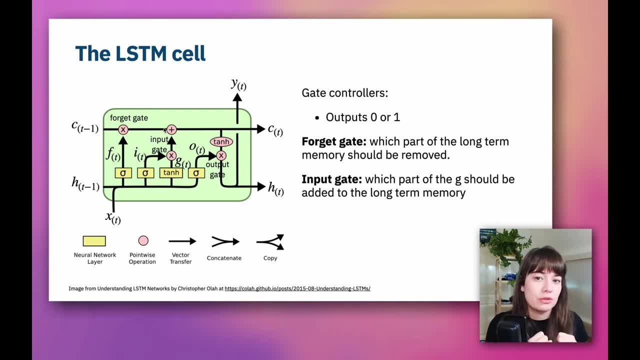 the long term memory. So we're deciding- OK, actually this piece of information is going to be important to remember later- And in the output gate we decide which part of the long term state we need to extract from the long term state right now and use as an output, either, as in the hidden. 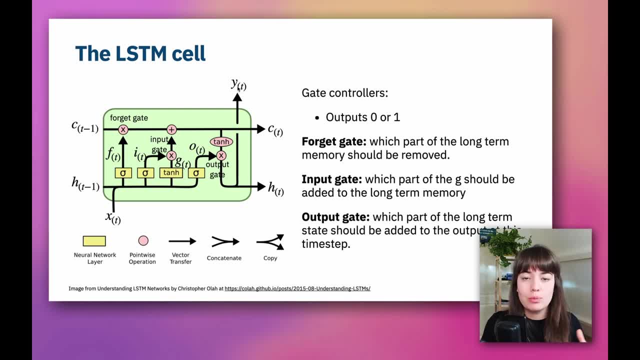 state to pass on the next timestamp, or as an output in this or as part of the output that we generate in this timestamp. So it sounds kind of complicated, even though it's sort of intuitive that there is one long term memory, one short term, shorter term memory, And then we either 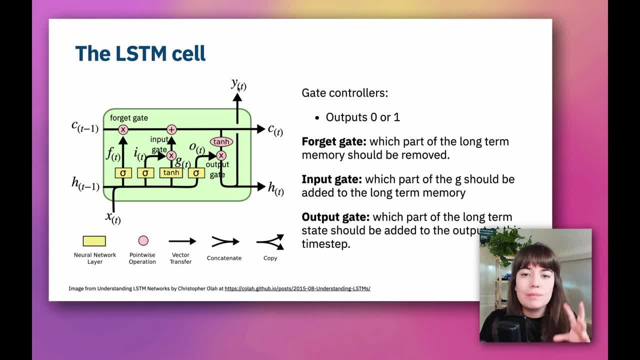 forget things from the long term. one either use it or add new things, And it's kind of confusing to understand. OK, well, how does this thing whole work? Why do we forget input? or how does the forgetting and inputting happen? But you don't have to understand everything behind it, You don't. 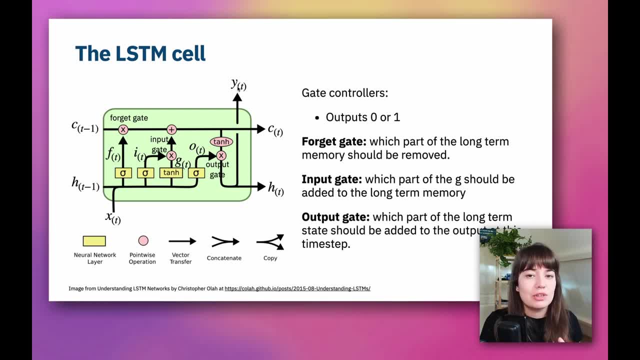 have to understand how it's all working. Basically, what you need to know is that it is working, and this is the intuition, And I think that will get you where you need to go, So you don't have to obsess over how this whole works. 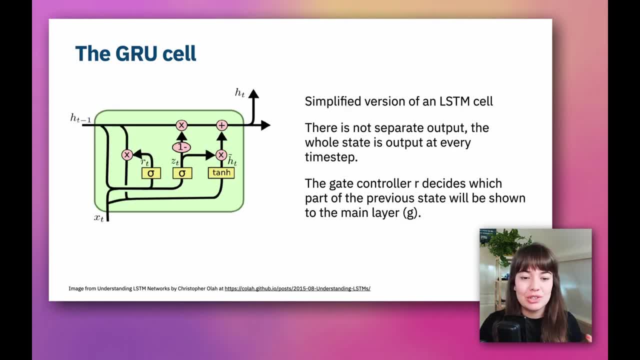 So another different kind of cell that we have is called the GRU cell. GRU cell is basically like a simplified version of the LSTM cell. You know you have less things happening here. You do not have a separate output, As you can see the hidden state that is passed to the next timestamp and the output.